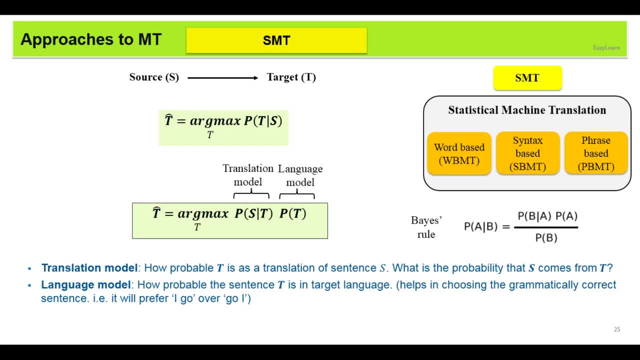 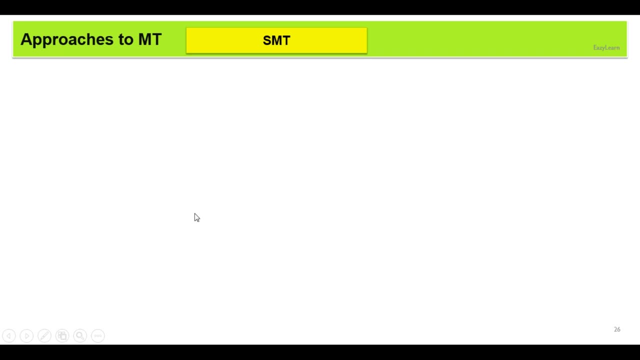 probable, or how correct the sentence is Grammatically, how correct it is, For example, it will prefer the sentence I go over, go I, And the decoder performs the search operation. That means this is argmax operation. Now let's see an example of this. So we have a French sentence. 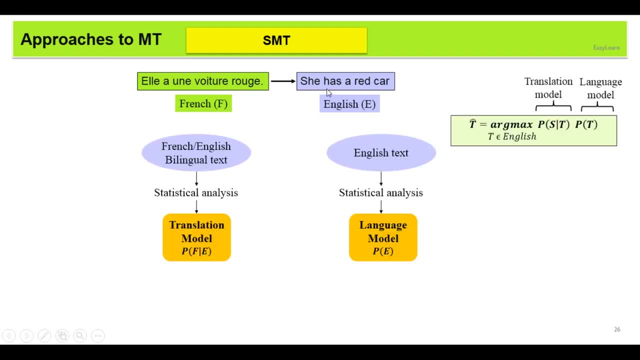 and we want to write a French sentence. So we have a French sentence and we want to write a French sentence. Well, we have a French sentence and we want to write a French sentence and we want to write the English word on this one value. 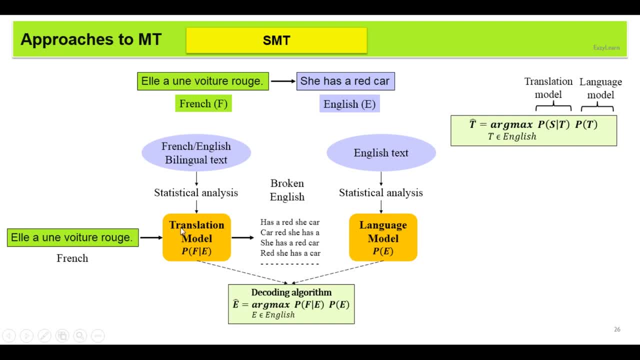 This hunt. So now we have to'm using the translation moral. We have a French to English bilingual corpus. from that we launch the parameters, or the translation model, And from the target language, English, we learn the language model. So, given a friend sentence, the translation model produces a set of candidate translations. 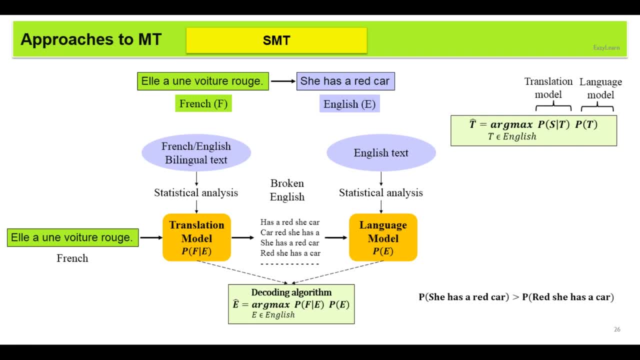 and we trust the language model, helpless to choose The language terms that the world's the right one or the most natural one. for example, if you see here, the probability of she has a red car will be more than the probability of red she has a car, because the first one is a more natural sentence in English. that's why. 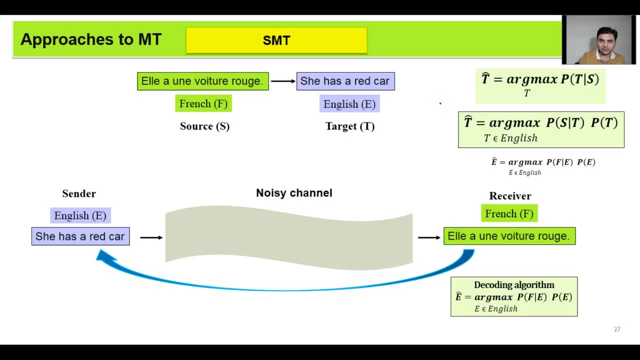 it will prefer the first sentence. all right, but there is a interpretation problem here in the state from our formulation. you were interested in the conditional probability of T given s, because we were given s, but in the second formulation we are interested in the probability of s given T, but T is. 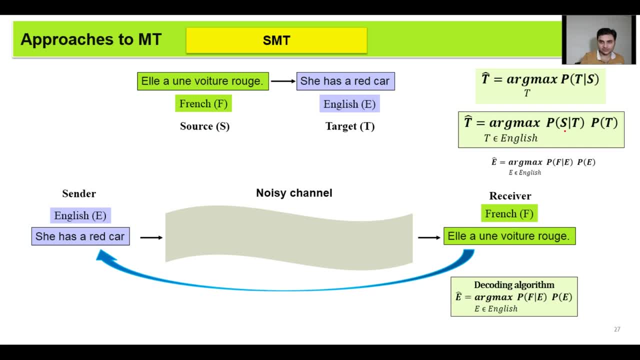 not given to us. so what is the interpretation of this? so to understand that, let's look at the noisy channel model first. so in the noisy channel model, we assume there is a sender who sent the English message through a noisy channel and that channel corrupted, or we consider terms translated that English message into: 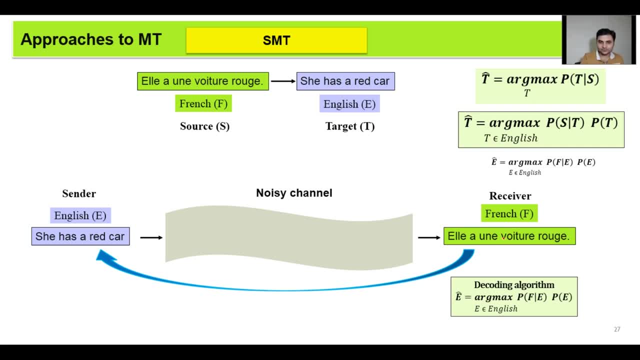 the French sentence now being at the receiver end, we need to guess the original message, which was in English. now our decoding algorithm will iterate over a set of possible English sentences which could be the original message, and that's what we are doing here in the argmax now. whatever sentence we consider in English, that also has 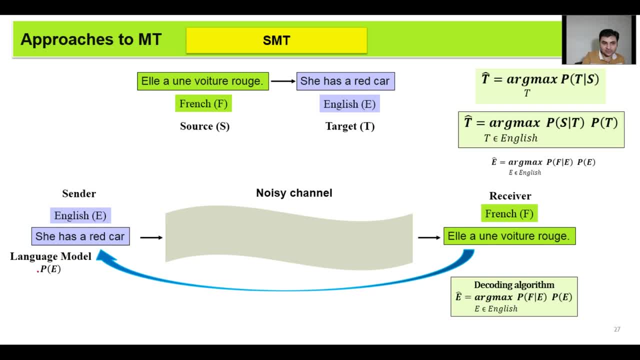 some probability of being in English. that is given by the language model P of E here. now, when the sentence passes through this noisy channel, this channel has a probability of translating or corrupting each word of this English sentence into the French. so that's how we get the French sentence now, if you. 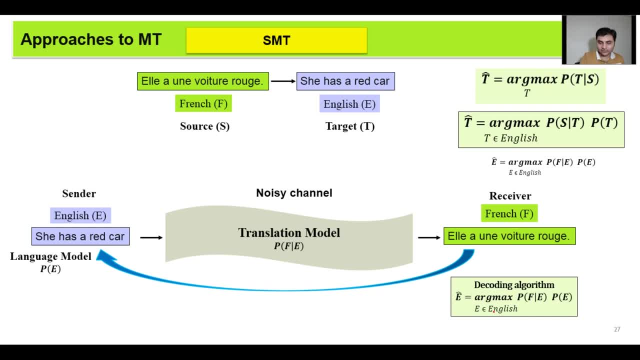 multiply this sentence with the English sentence, then you get the French sentence. so that's how we get the French sentence now. if you multiply this probability and this probability, we'll get the probability of this English sentence to be the original sentence of this French sentence F, right and now. 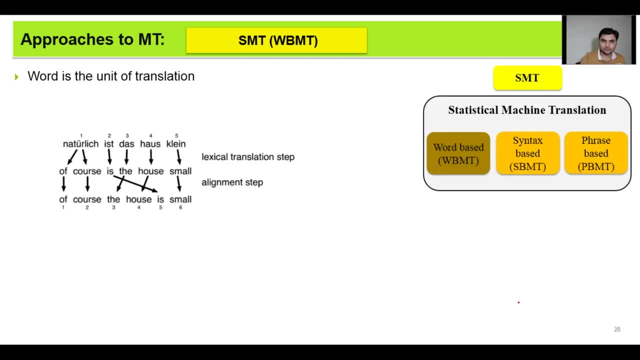 these probabilities will make more sense to you now. there are three approaches of this statistical machine translation. so one is first, one is a word based machine translation. in the word based machine translation there are two steps. the first step: we translate each word was source sentence to the target language and once we are done with this, we use the 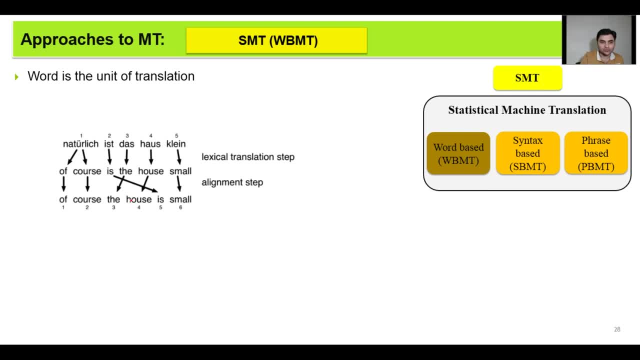 alignment model to align the words and form the proper sentences. there are more details to it, but I will not be spending more time on this. I will be spending more time on the neural machine translation. the second: we have the Syntex based machine translation. so in the Syntex based machine translation, 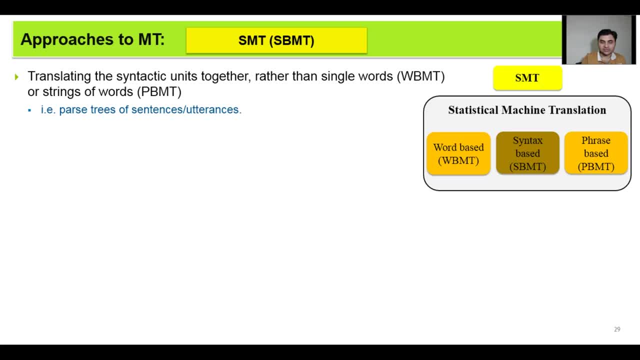 we do not translate the single words, rather we translate the syntactic units. now, let's say we are translating from English to Japanese. so first we created past tree of the English sentence and then we converted, and then we convert this past tree into the grammatical according to the grammatical structure.